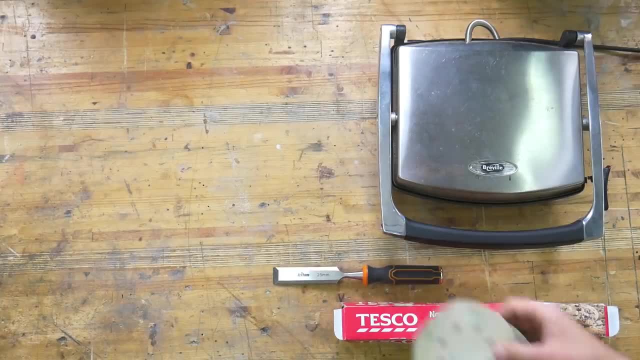 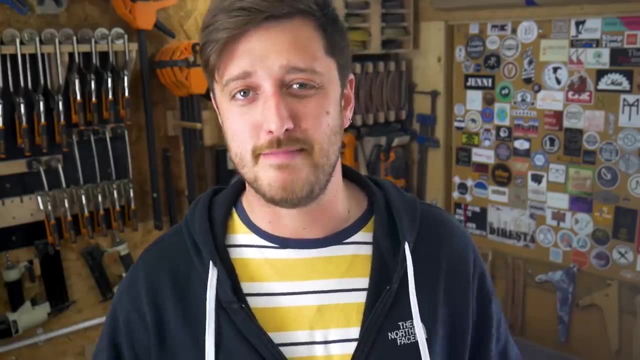 from sticking to the press, a chisel or a sharp knife to clean up the rough edges, some sandpaper in a range of grits, a drill, a coping saw, some clamps and a good pair of oven gloves. Our favorite are silicone oven mitts, as they don't. 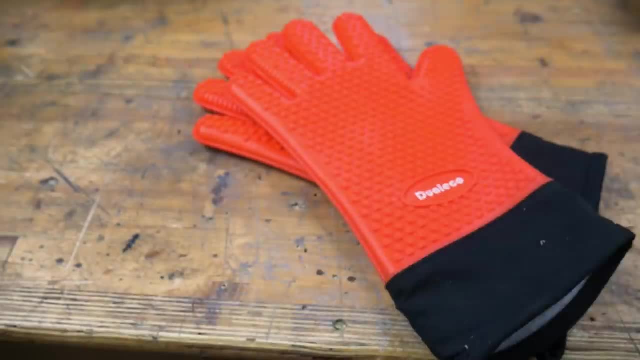 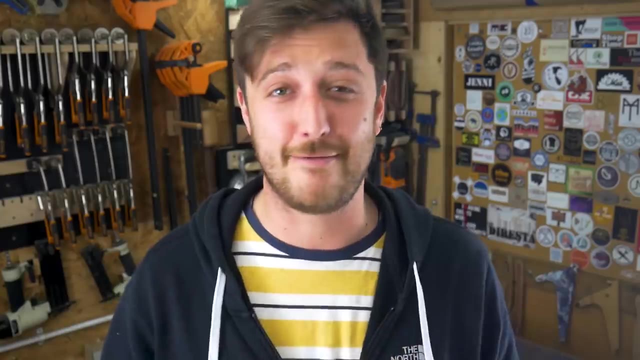 stick to the melted plastic. So we know what some of you might be thinking: Won't melting plastic release toxic fumes? For some plastic, you might want to use a heat gun For plastics. yes, but HDPE is different. As long as the plastic you're. 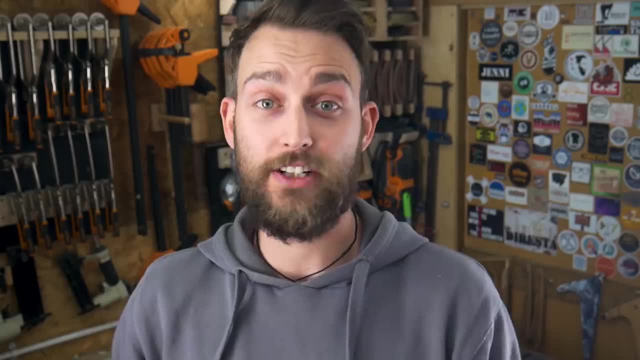 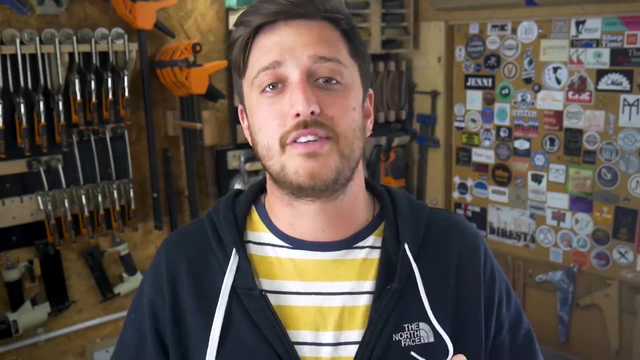 melting is clean and you don't go above the burning point of 180 degrees C, then nothing harmful will be released. However, if you are concerned about a rogue piece of dirty plastic getting into the mix, or if you're doing on a larger scale, you may want to invest in a respirator. If you do, we recommend a 3m respirator with. 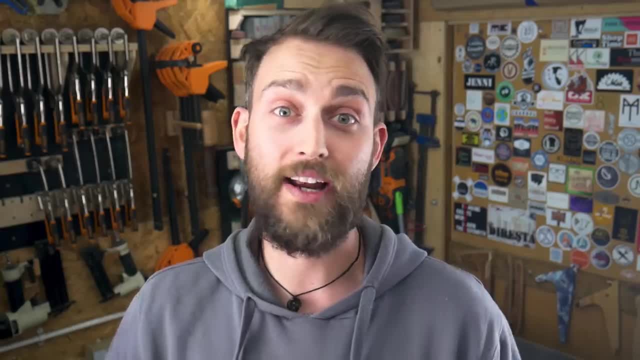 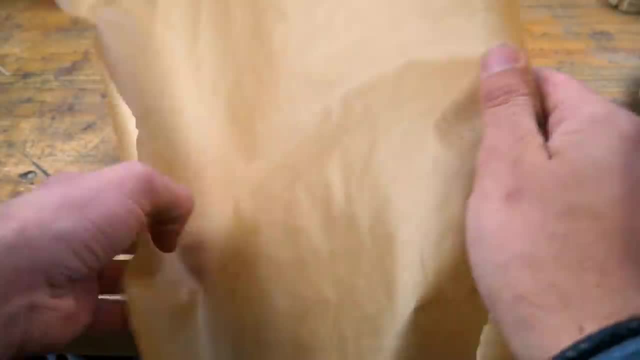 a set of ABEK1 filters, which are designed for non-organic vapors. So once you've grabbed your panini press, you'll want to line it in some way to make sure it's non-stick. Baking paper works great. however, if you're doing this regularly. 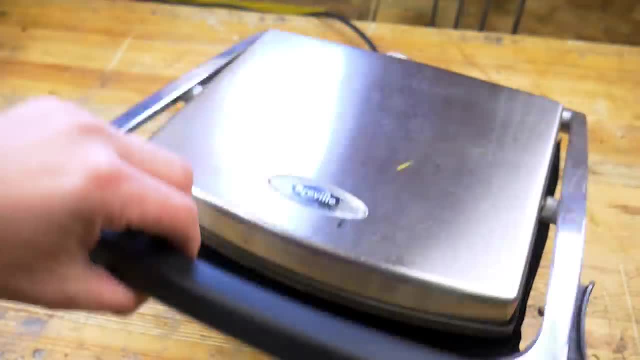 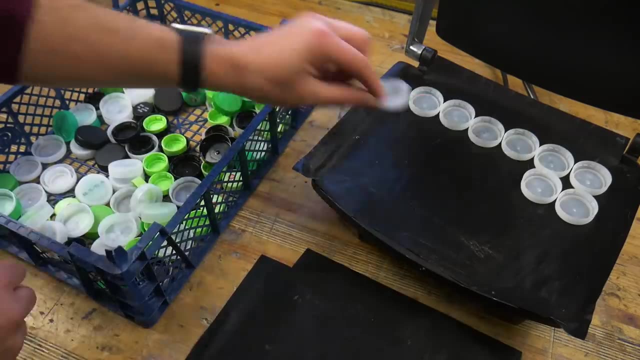 you may want to pick up some Teflon baking sheets, as these last a lot longer. After your press is warmed up, you'll want to start loading in your plastic. If you're using lids, you want to make sure these are top-down to avoid any air. 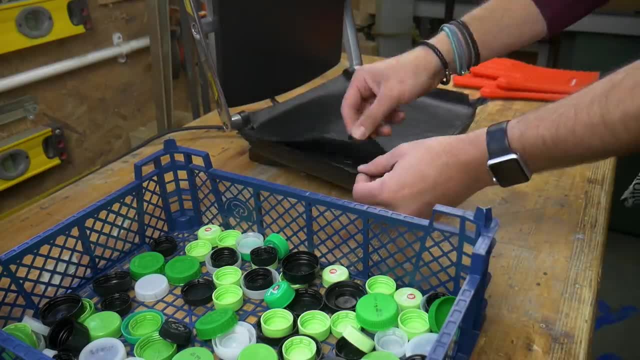 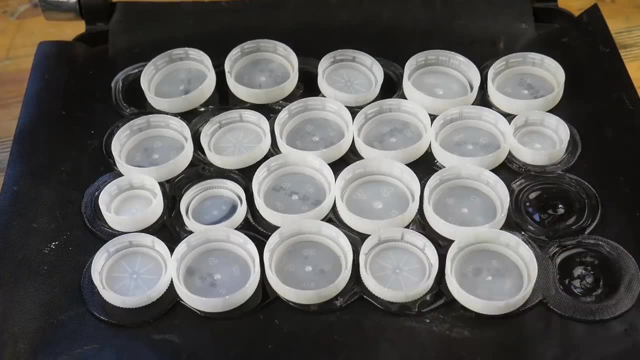 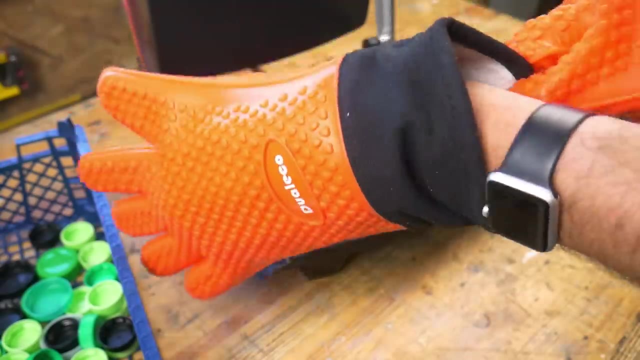 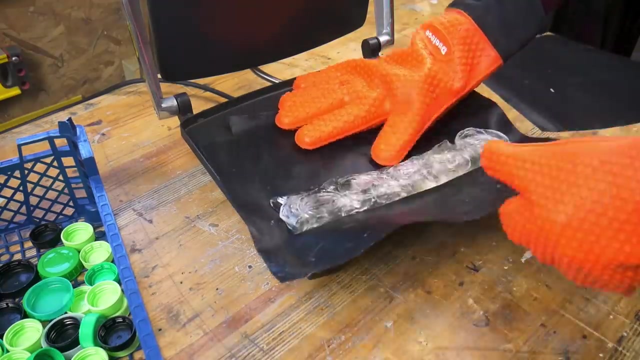 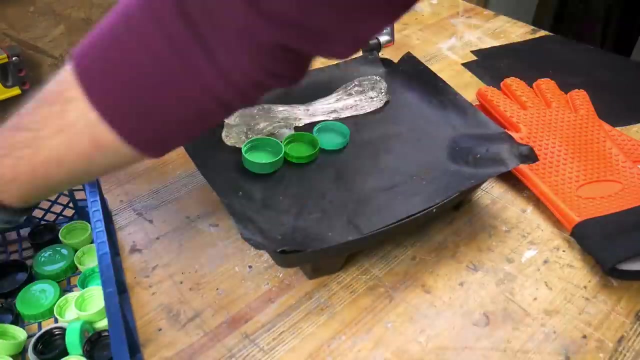 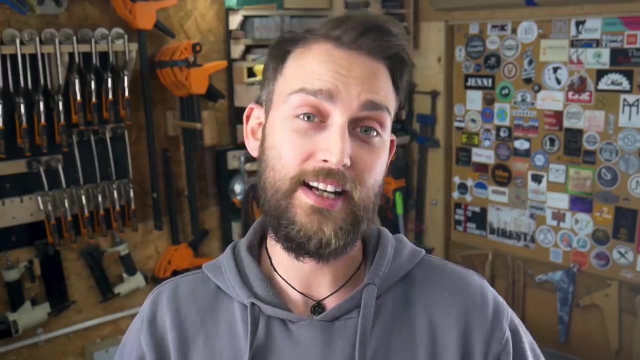 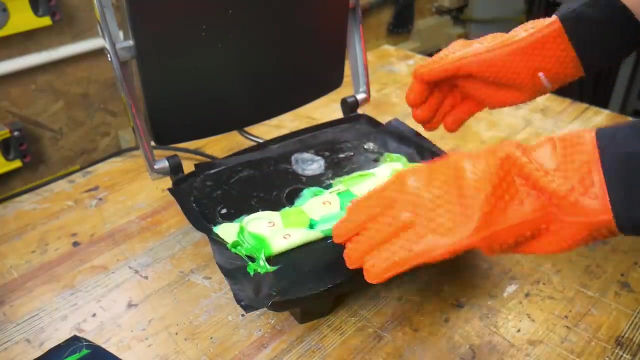 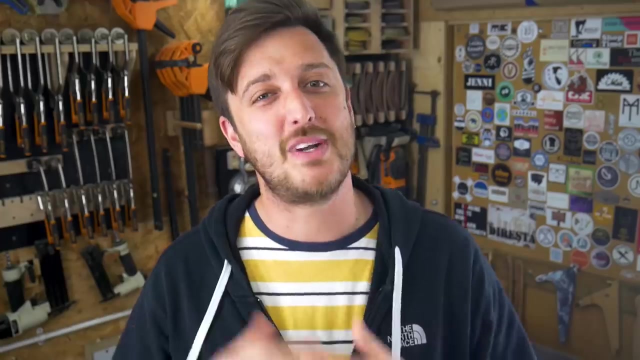 being trapped. You'll notice that we like to keep our colors separate in the initial melting phase, as this gives you a little bit more control over the marbling patterns you can achieve. The twisting and folding throughout ensures that any air bubbles are worked out of the plastic as well as giving you that striking marble pattern. 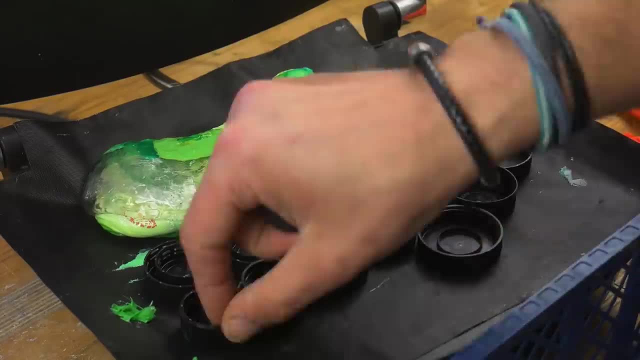 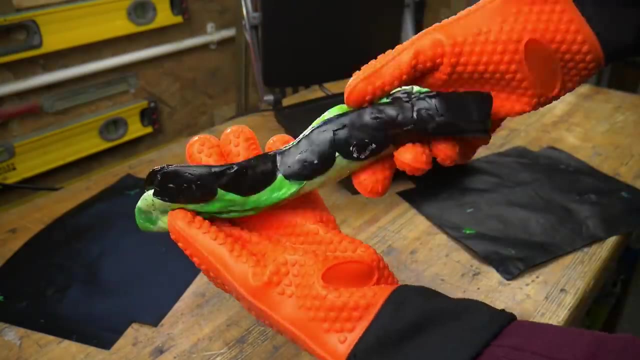 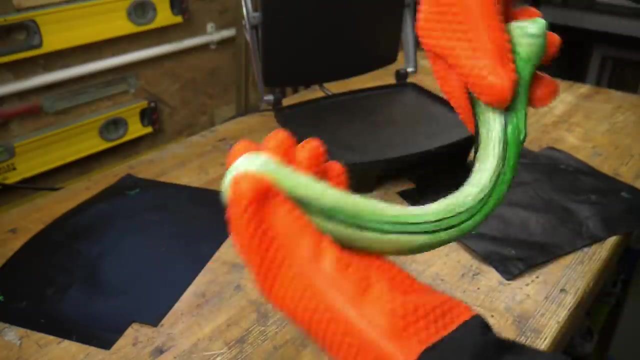 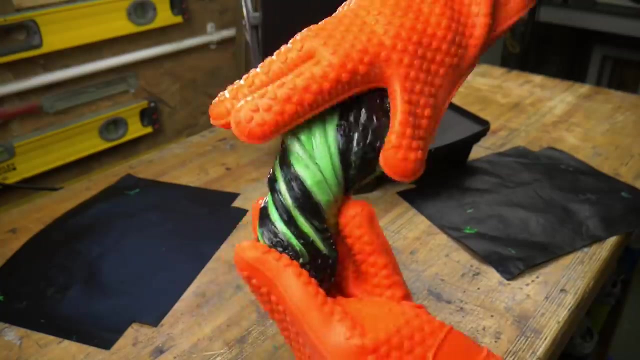 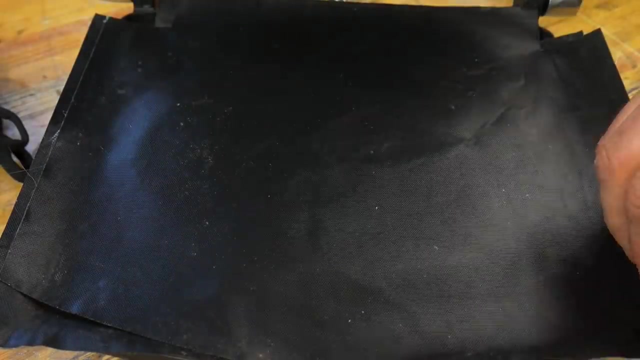 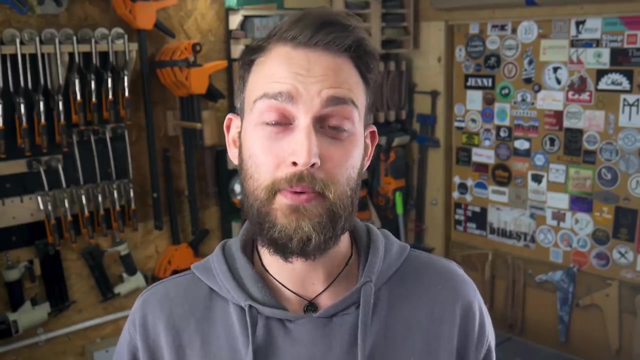 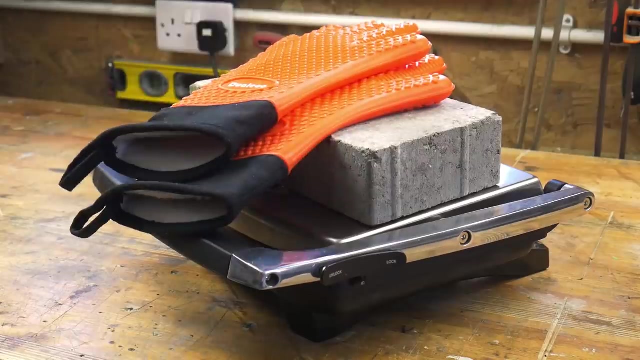 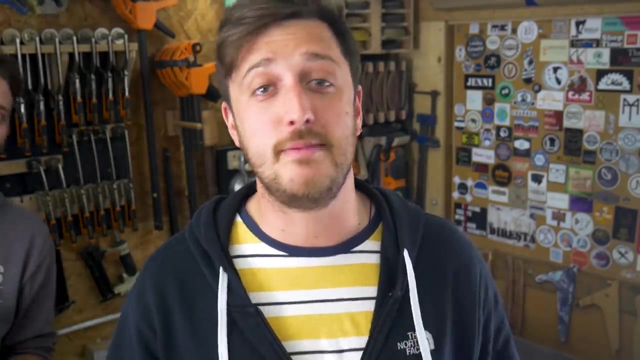 If you like this video, please give it a thumbs up and don't forget to subscribe to our channel for more videos like this. Thanks for watching, and I'll see you in our next video. Now we're going to show you how to make some coasters out of your new sheet material. 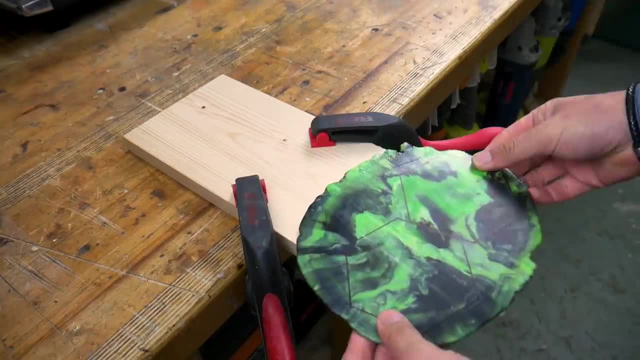 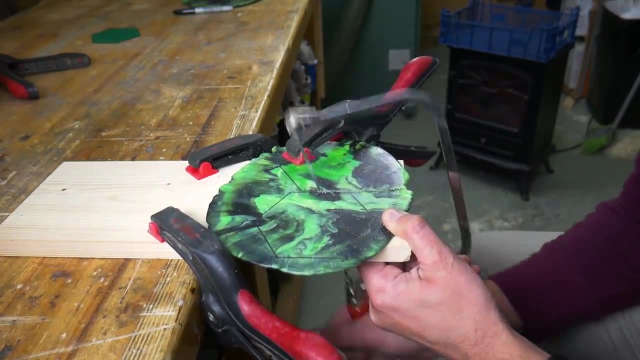 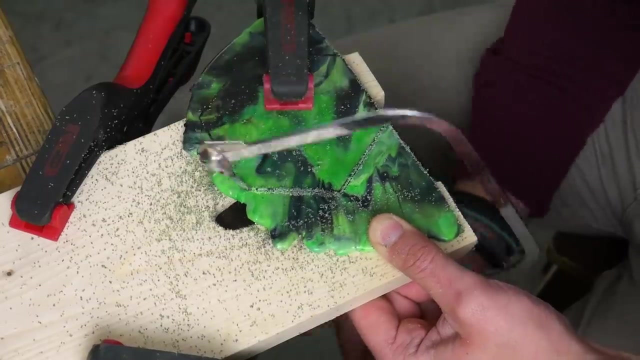 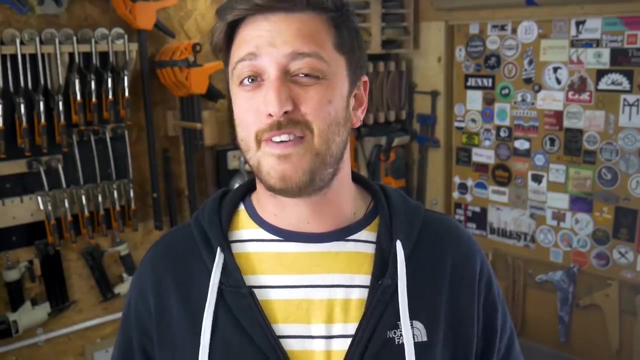 Simply mark on your desired shape, clamp it down and cut to the line. A coping saw is about as simple as you can get, but feel free to use anything you have to hand. You'll then want to tidy up those rough edges. A sharp knife here works well, but we find a chisel. gives that a little bit more control. 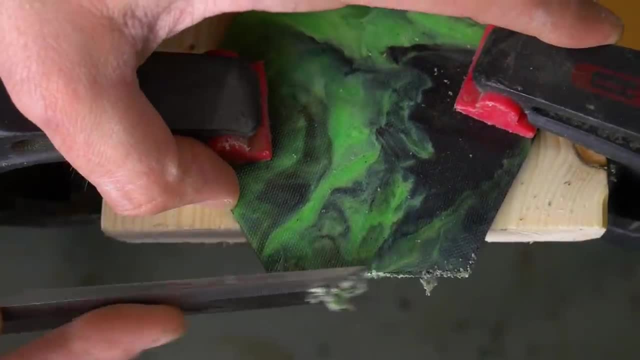 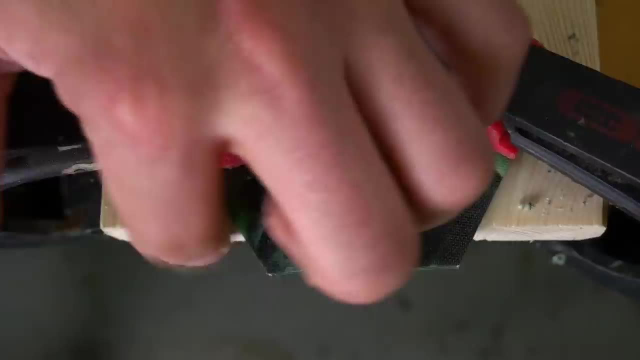 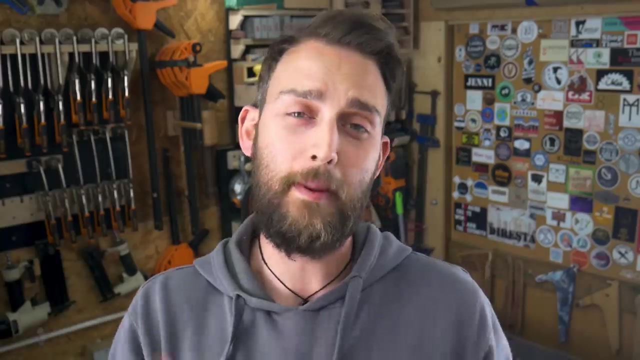 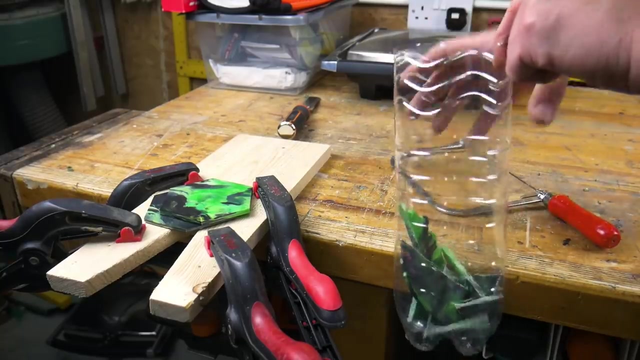 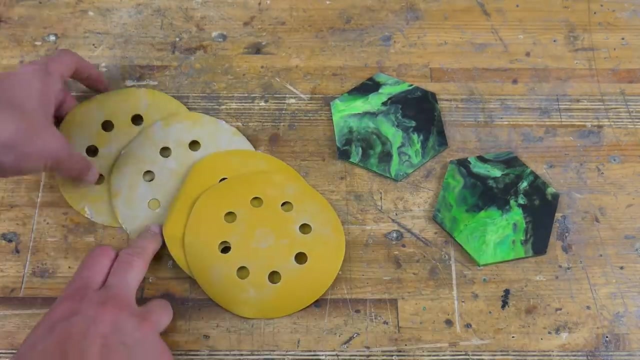 As always, the fabulous thing about working with recycled plastic is that you can save all of your offcuts for use in future projects, So you could absolutely leave it there. However, we wanted to give ours a sand up to 400 grit, just on the top surface. 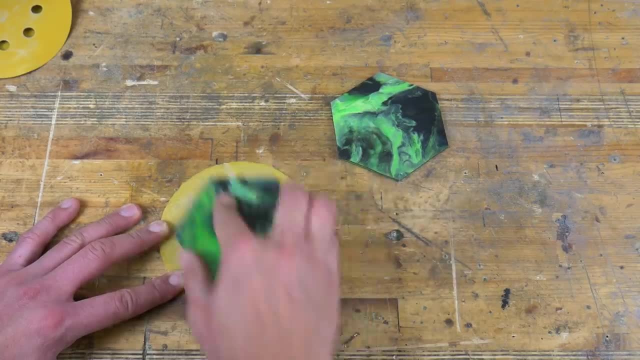 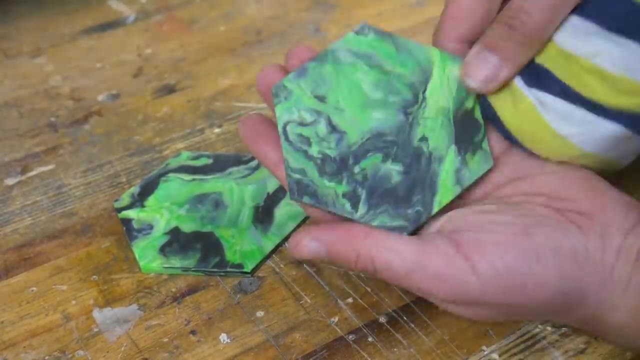 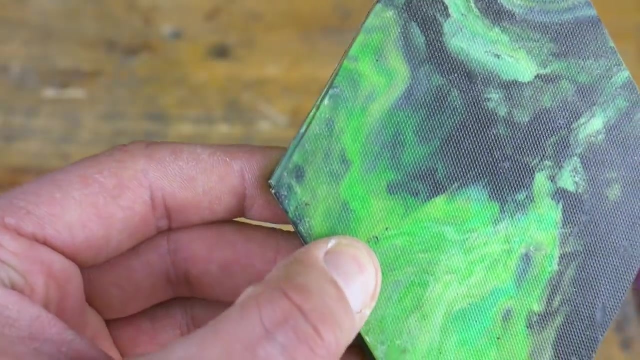 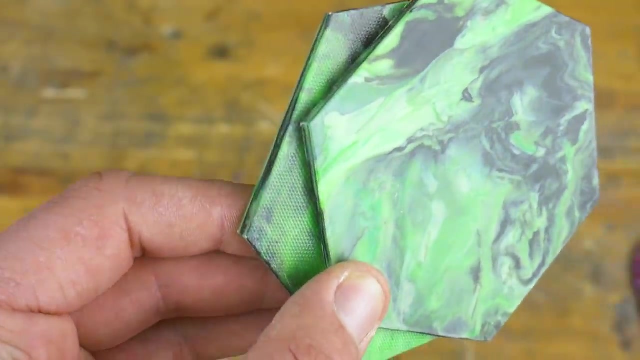 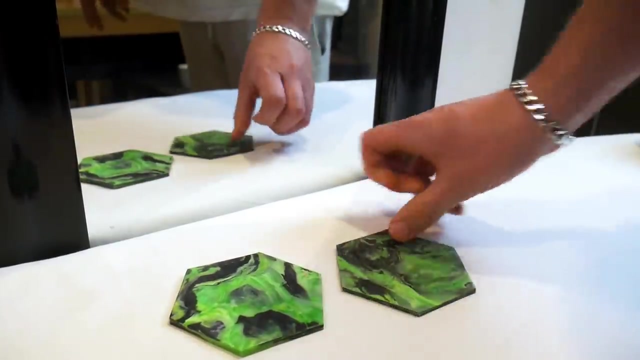 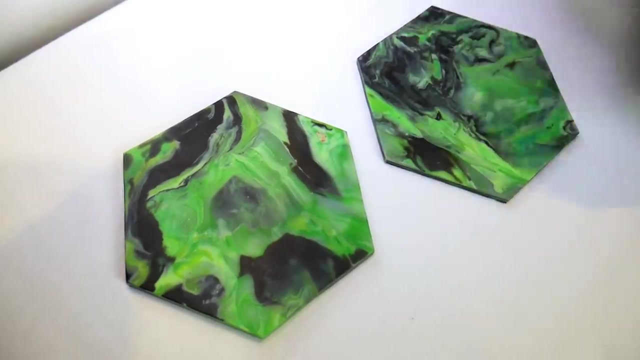 Be aware that sanding will create microplastics. To combat this, we use a dedicated dust extractor so that we can clean up after ourselves and reuse it later. So let's get started. Next up, we're going to make a pendant. 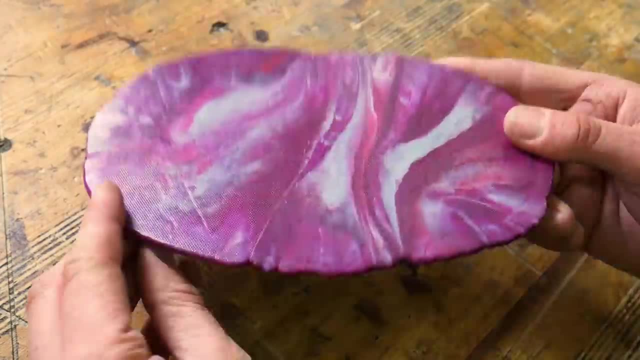 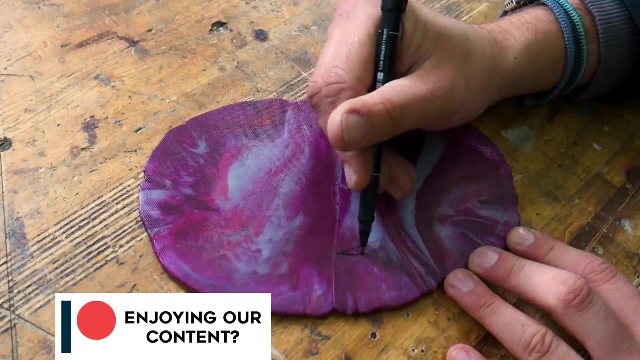 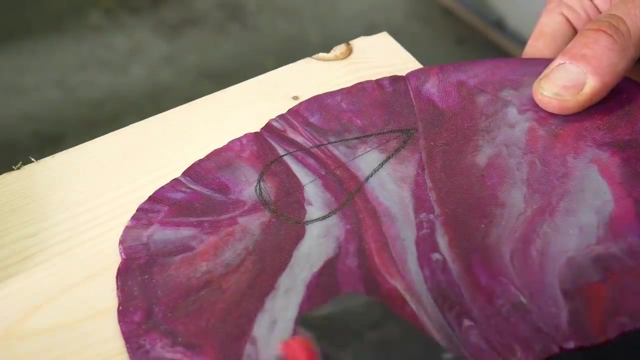 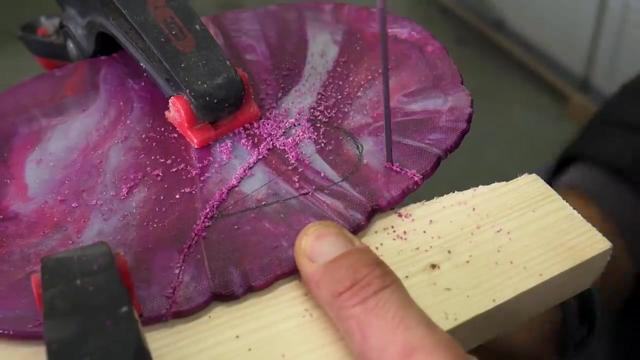 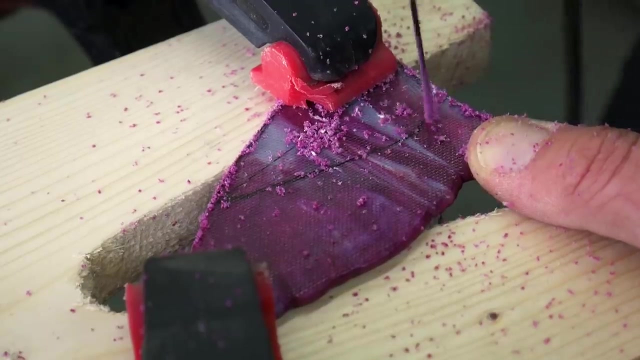 Using the same technique as we did before. we melted another slab in a different colour before cutting it out and shaping it Until it's all melted. Now we're going to use the same technique, but we have to do it differently. We're going to start it off with a bit of mud. 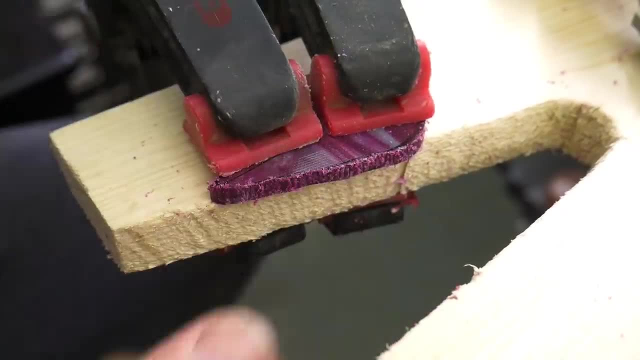 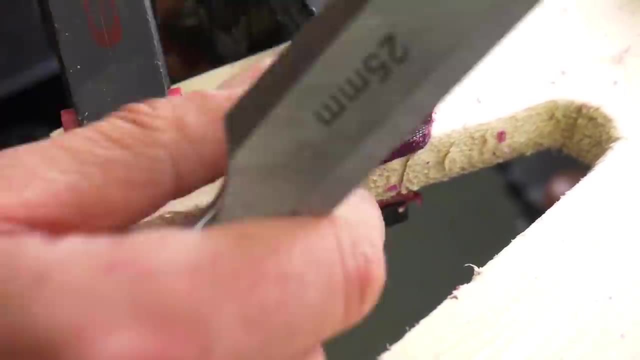 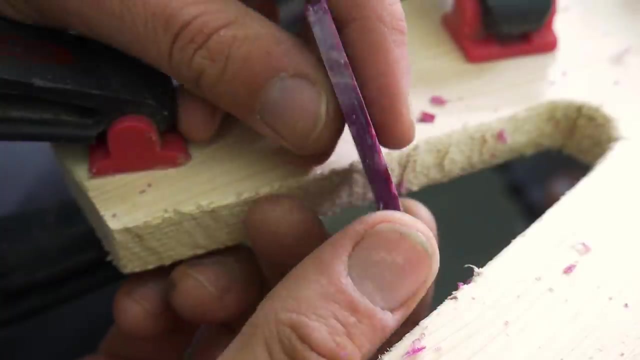 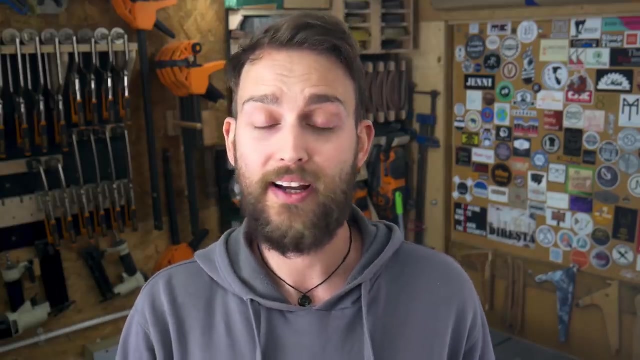 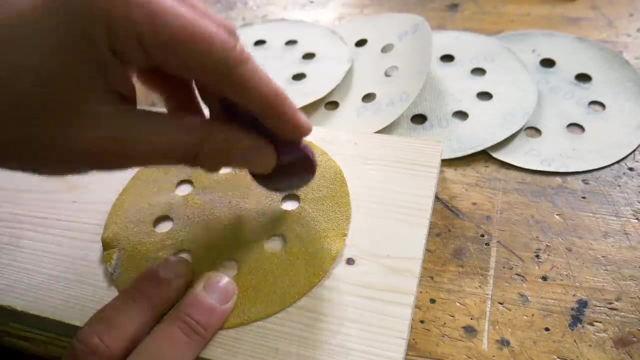 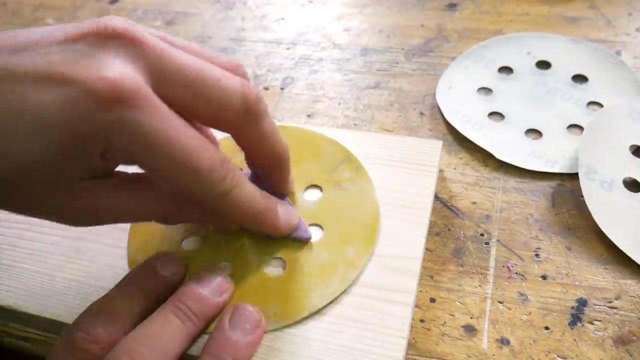 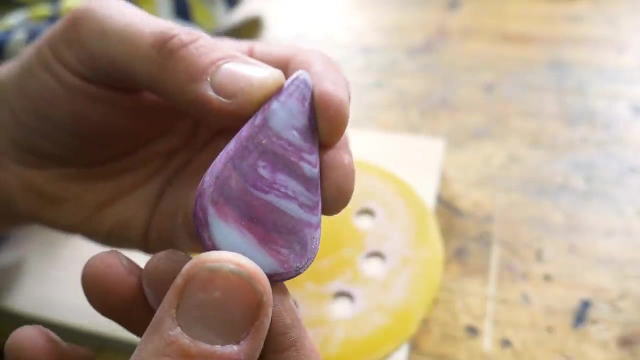 1, 1.5, actors, 2, 1.5, второй, 3, 4.. Since this is for a piece of jewellery, we wanted to give it a slightly nicer finish, so we started hand sanding at 120 grit and took it all the way to 600. 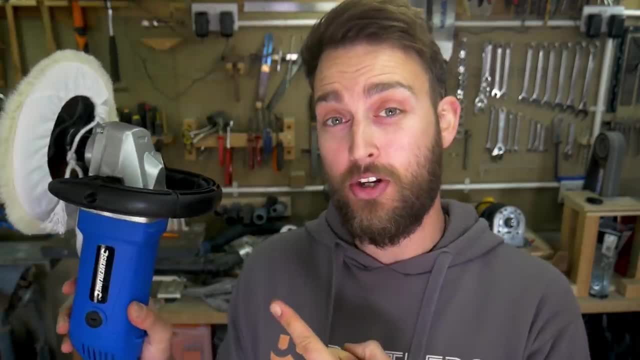 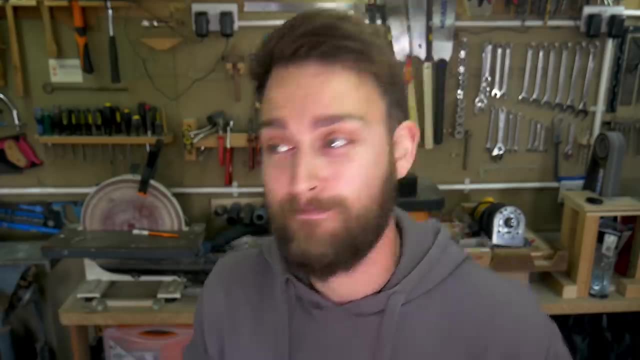 Now, our favourite way to polish recycled plastic is to use one of these car polishing tools, but since this is a limited tools project, we're going to assume you guys don't have one of these and we're going to go find something else that might work instead. 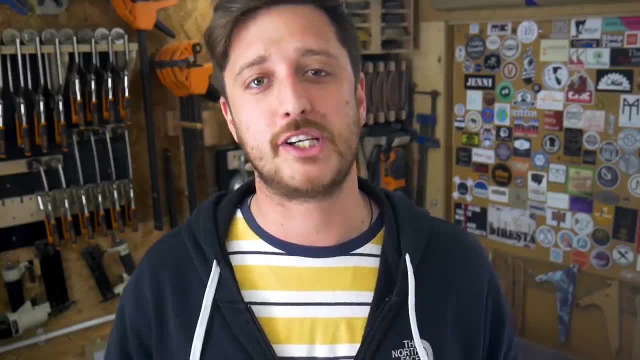 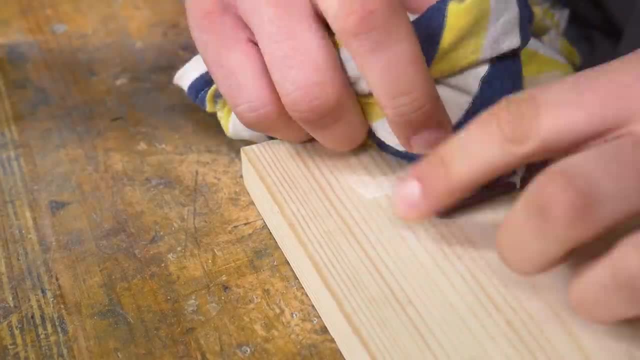 Any type of polish will do the job to give it a bit more of a shine. so we razed our kitchen cupboard and found a few things that could work. We prefer to use a polish over a wax, as the wax would sit on top of the plastic making. 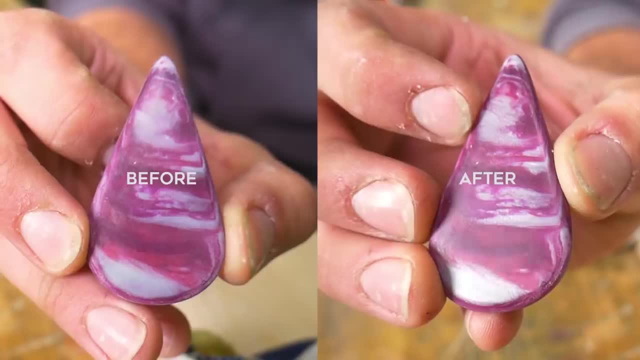 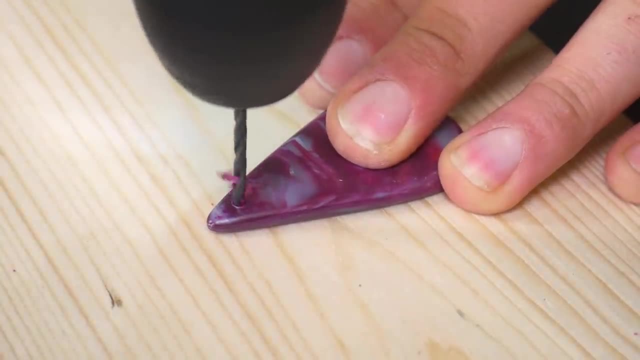 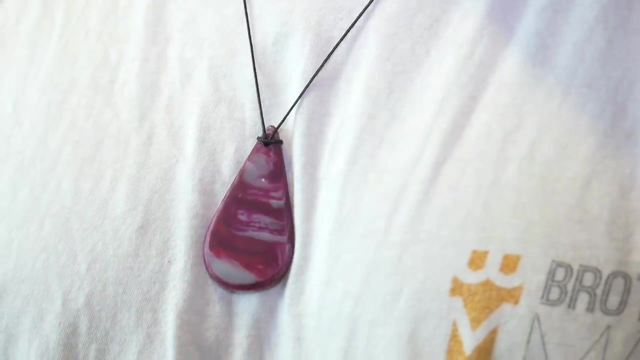 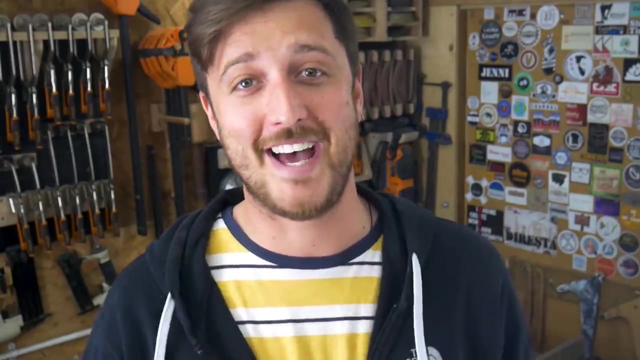 it much harder to recycle in the future. Just before we show you how to make our third and final product, we just want to take a quick moment to talk about this video's sponsor, Skillshare. Skillshare is an online learning community with thousands of inspiring classes for creative 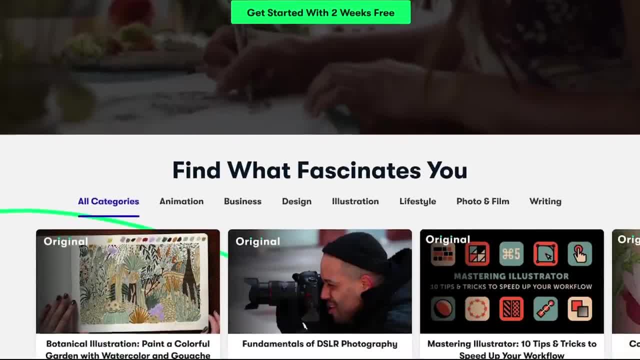 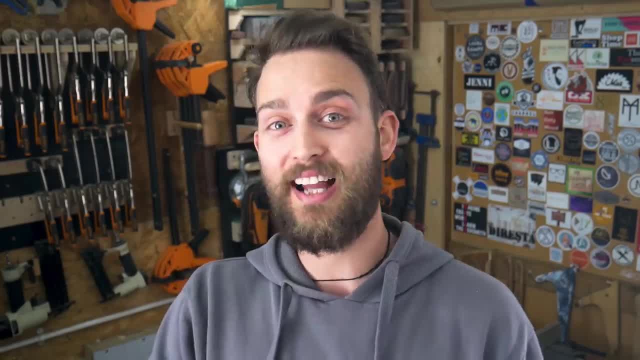 people. It enables you to explore new skills, deepen those existing passions and just get lost in your creativity. Some topics we've got on our watch list include sustainability and home recycling, as well as presenting to camera and how to make engaging videos. One class we've been really enjoying recently is building an Etsy shop that sells by Parker. 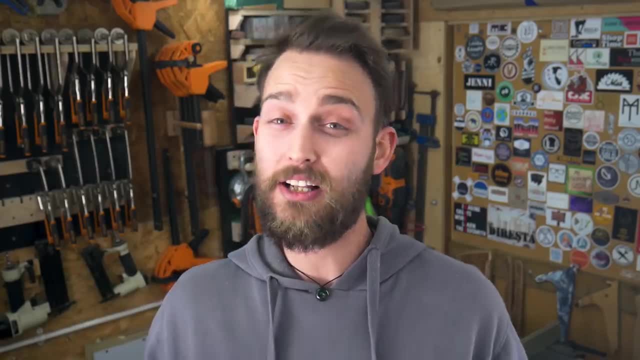 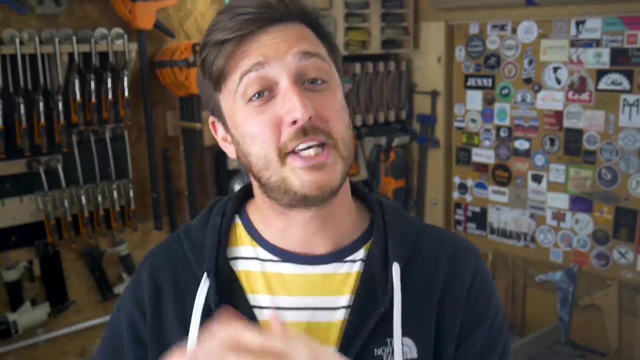 Gard, Since we recently launched our online shop and Etsy store. this class was fantastic at giving us tips on how to make us more discoverable so more people can find us and see our recycled plastic products. It's curated specifically for learning, meaning there's no ads and they're always launching. 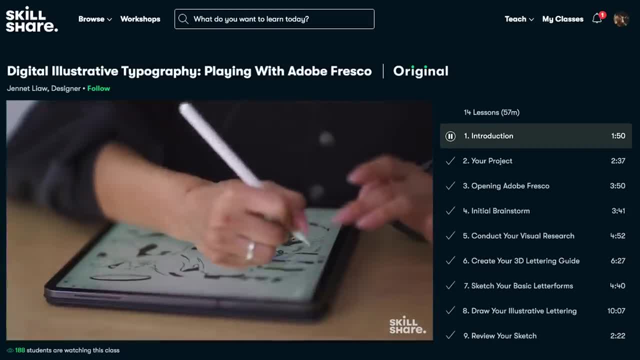 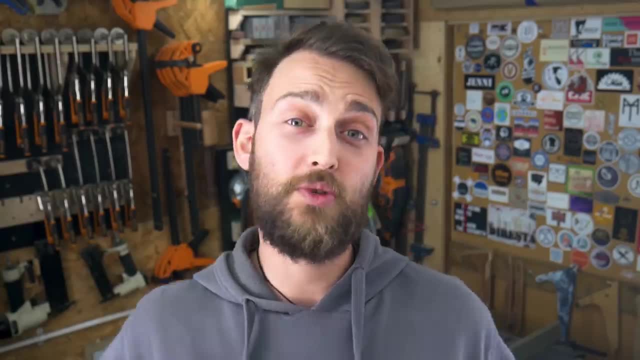 new premium classes. This helps you to stay focused and follow along wherever your creativity takes you, And you get all of that for £7 a month, which is just less than $10 with an annual subscription. Also, the first 1000 of our subscribers to click the link in the description will get 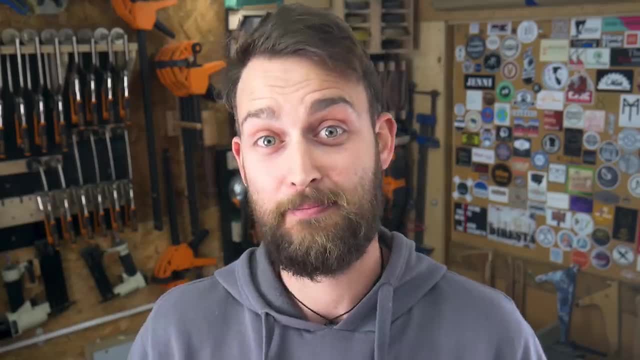 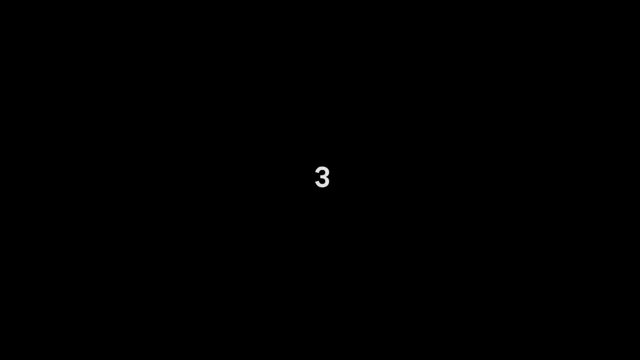 a free trial of Skillshare premium so you can explore your creativity. So a massive thanks to Skillshare for sponsoring this video and supporting the channel. Now back to melting plastic. The third and final product we're going to show you how to make is a simple keyring. 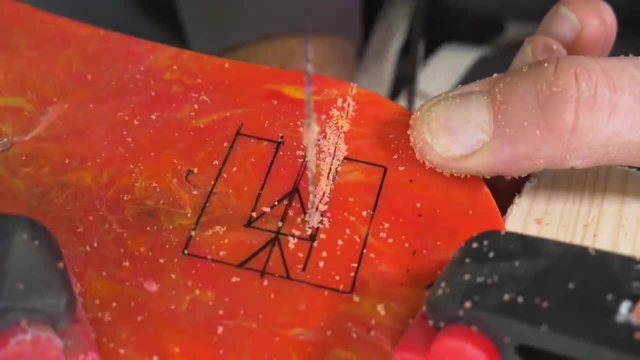 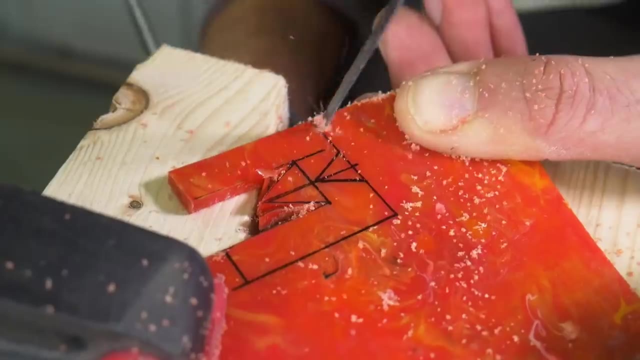 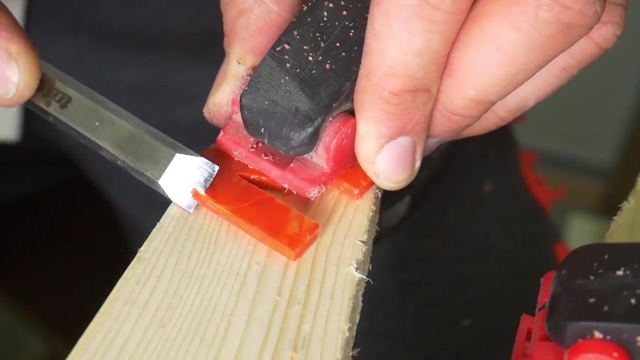 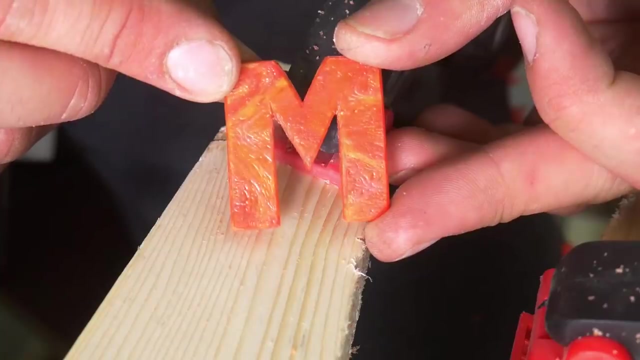 Once you've decided on your shape, you should need to follow the same steps as before. Since this is just a keyring, we didn't want to sand it in any way, but we did want to have a slightly smoother finish, So we switched back over to the baking paper instead of the teflon sheets, as these don't. 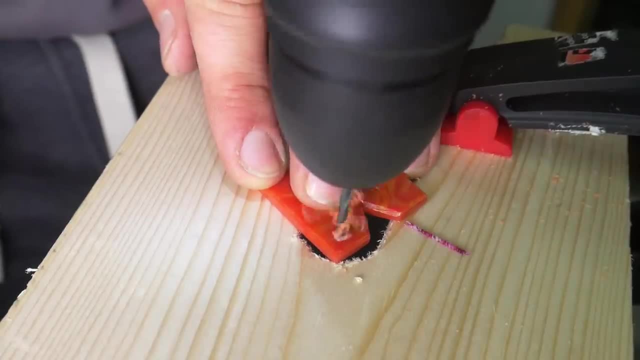 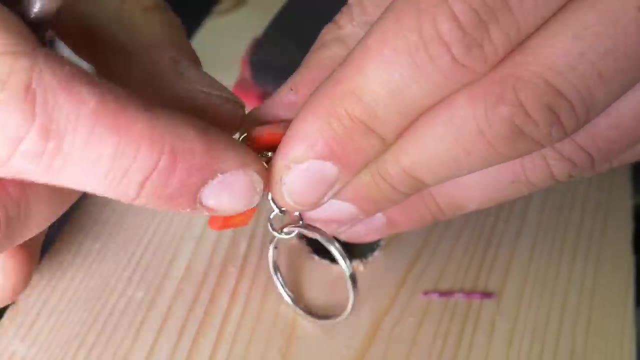 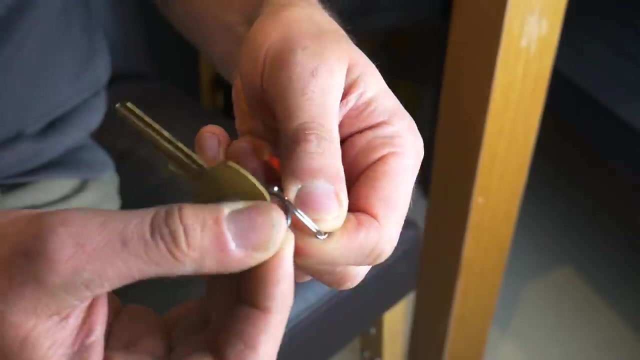 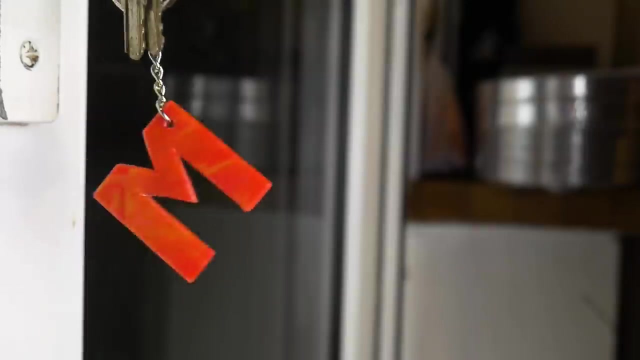 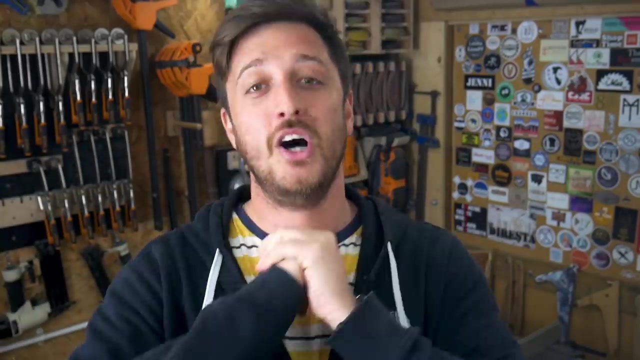 have a texture and it gives an overall smoother finish. So let's get started. So hopefully you've found that useful. we've popped links to everything we've used in this video in the description. Also, we just want to say a huge thank you to our wonderful patrons. 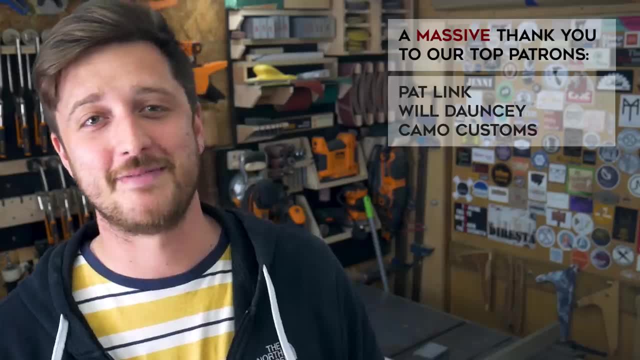 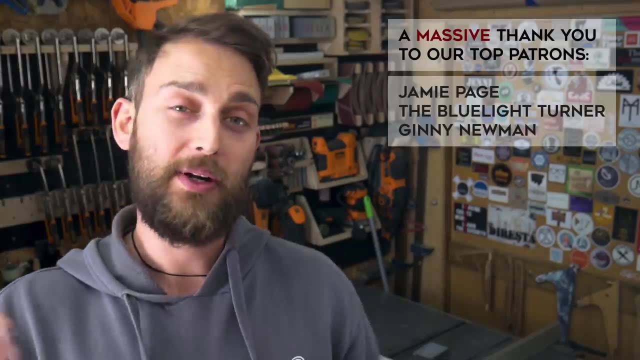 These guys massively help, support what we do and allow us to keep making videos, And if you're new to the channel, you may enjoy some of our other videos where we've used pretty much the same technique to make loads of other products. But if making is not your thing, then we also sell 100% recycled plastic handmade products. 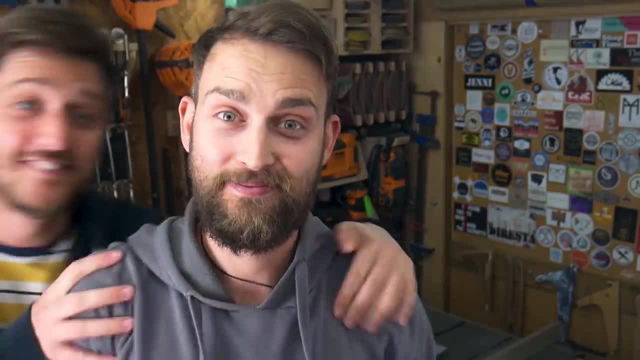 on our website and our Etsy store Links in the description down below. Thanks for watching Cheers guys. That must look quite shocking, but Jamie didn't know you were going to do that.